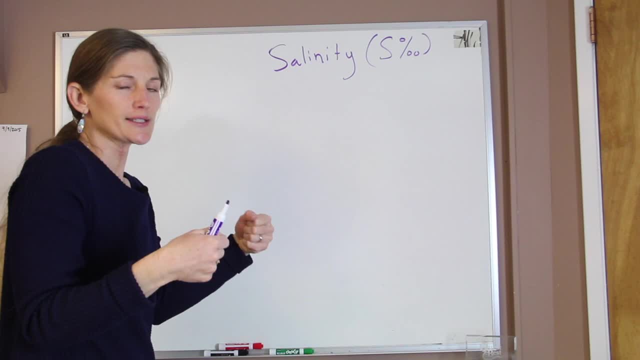 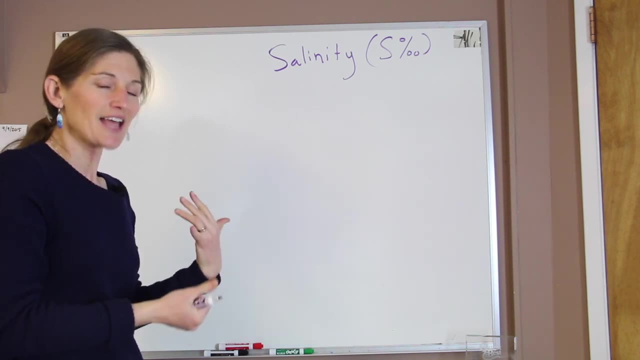 If we were to go and kind of take a whole bucket of seawater and scoop it up and let it sit and dissolve, evaporate away, and then take a look at all the residue that's left behind, we find seven major ions make up the majority. 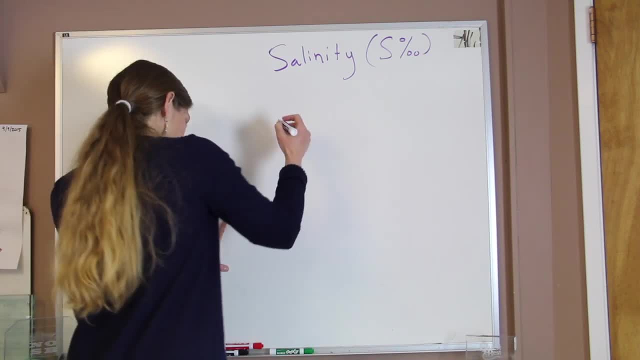 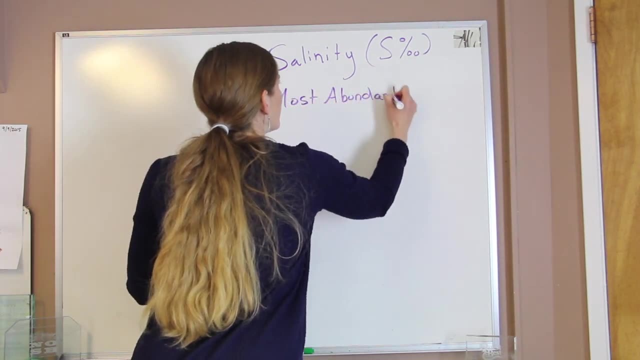 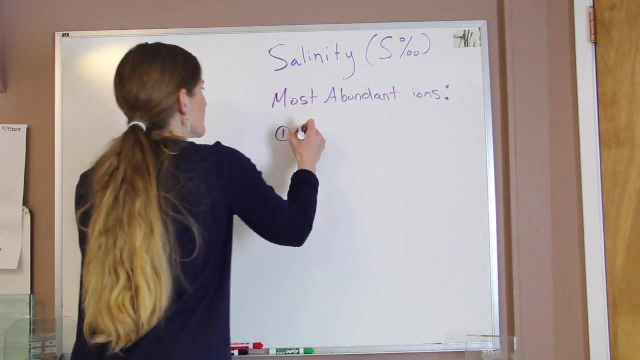 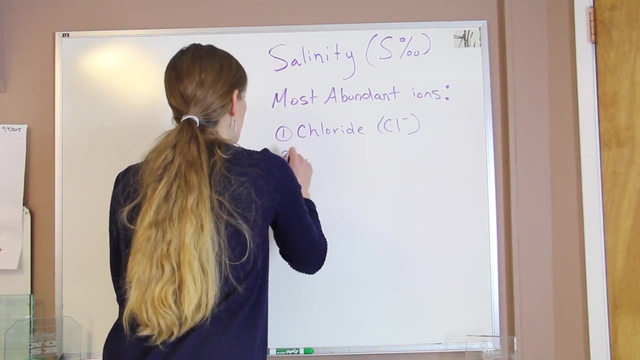 We find seven major ions make up the majority of those salts that we see in our seawater. So we'll write the most abundant Good things to know. The very first one kind of comes as no surprise- is our chlorine, And the second most abundant is our sodium. 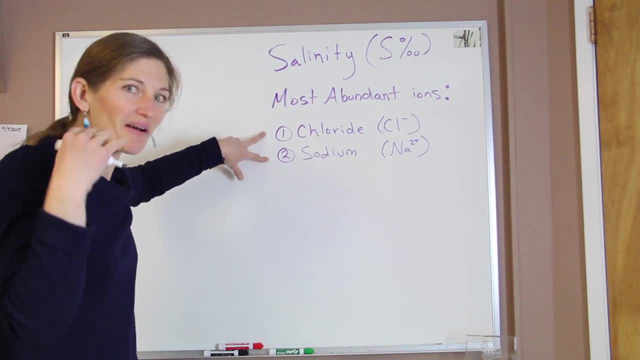 And what I find interesting is that, again, when we think about seawater, we think about salt. The top two ions that make up the most of those salts are sodium and chloride, which together, if the water evaporates away, these would combine together and make our table salt. 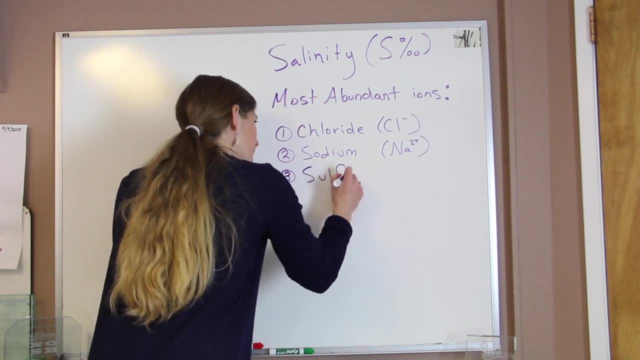 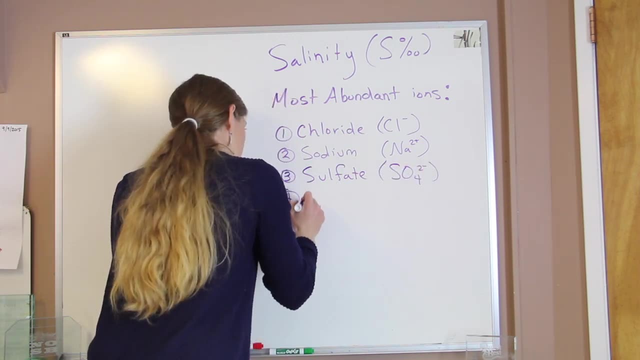 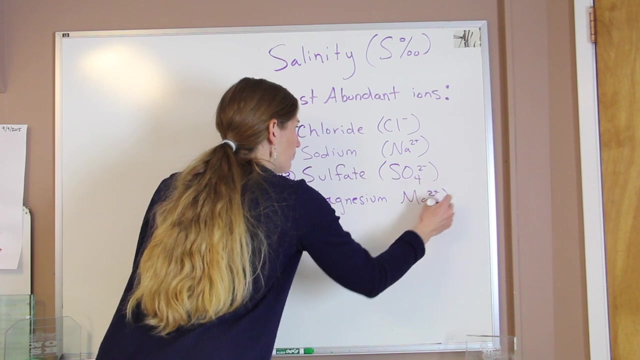 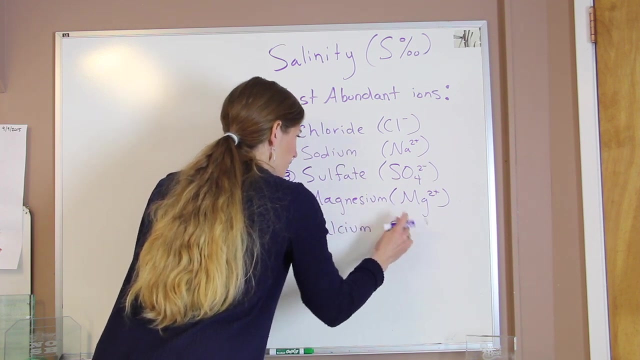 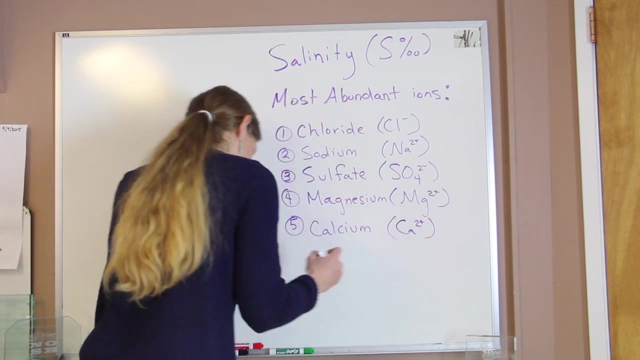 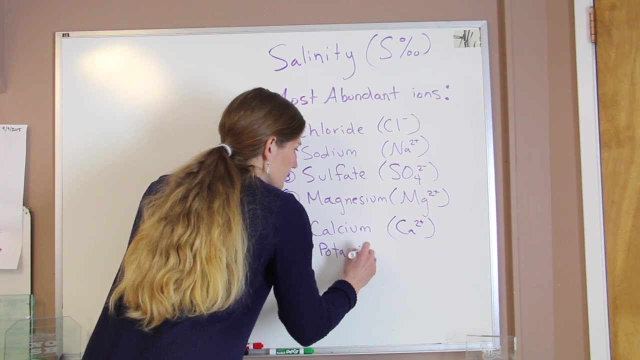 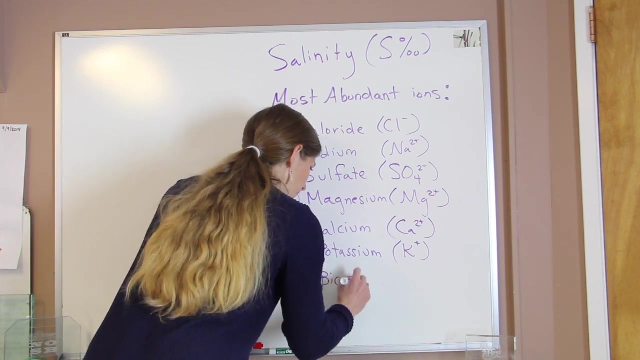 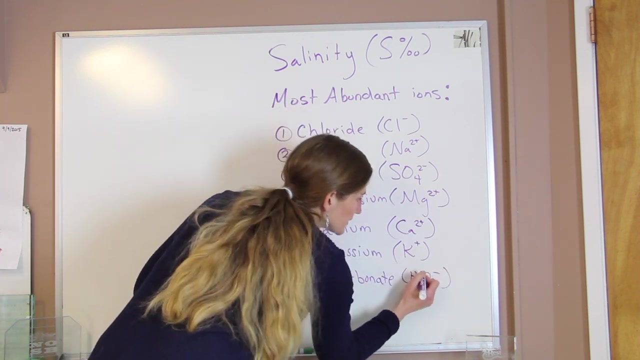 Okay, Number three on our list is our sulfate courage, followed by number four. We have magnesium, Calcium, Oops, And we have 6,, 7, potassium makes up number 6, and our 7th is our bicarbonate, which is H3, and that's a C, HCO3, and then it's got a negative 1 charge. 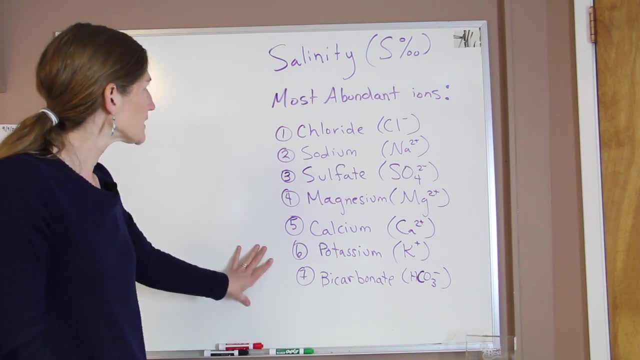 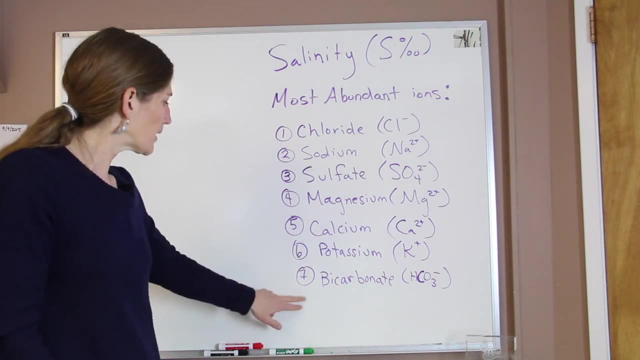 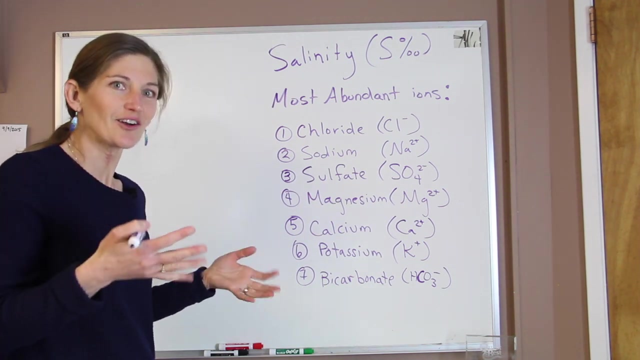 So all of these, this whole list, is the most abundant ions from top to bottom. There are other things, basically everything else. our trace elements would make up number 8, this is just different metals. all of these things that we find on our Earth are present in our oceans at very, very tiny amounts, less than 1%, so they're not listed here. 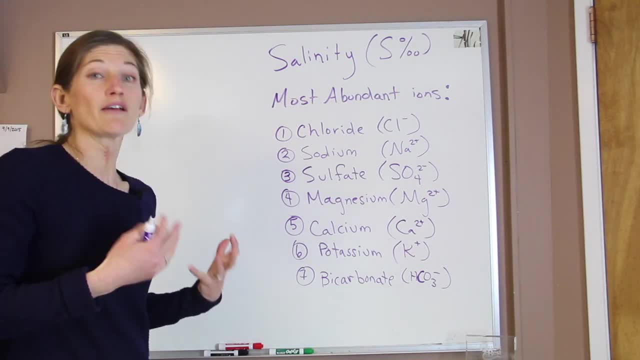 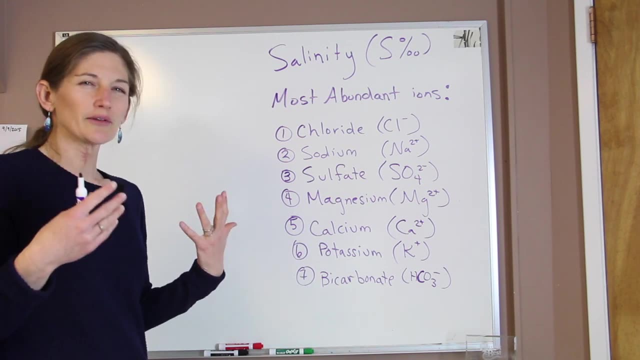 Now, when we go and we start to look at all of these things, the big question is: where do they all come from? So when we think about the oceans and we think about kind of what goes into it, we can really start to see some things. 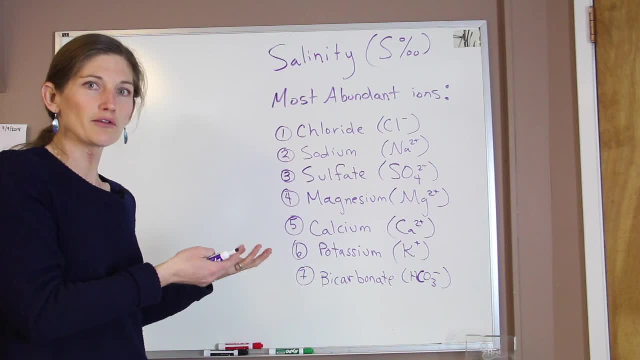 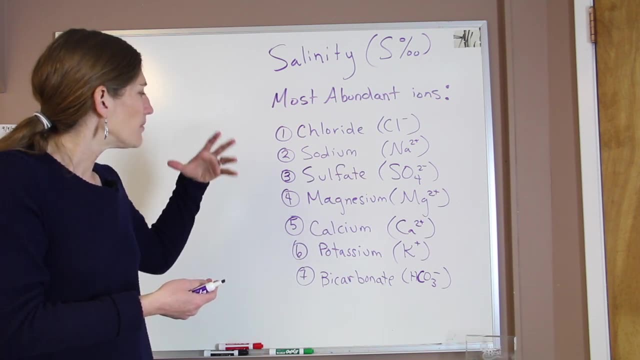 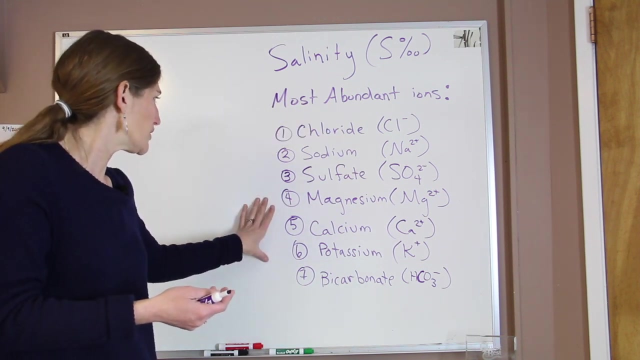 We see rivers running down the Earth and going into the oceans, So river inputs are one place that we do see these ions coming from. As the water flows over the land, it will start to weather the rocks, and then from those rocks we create some of these ions that go into our oceans. 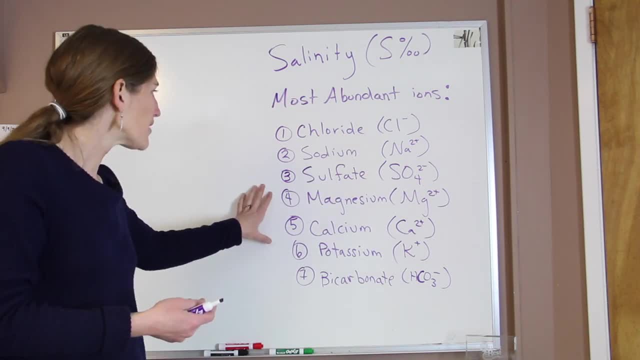 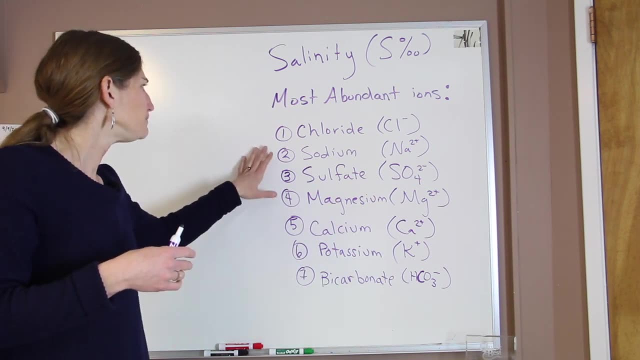 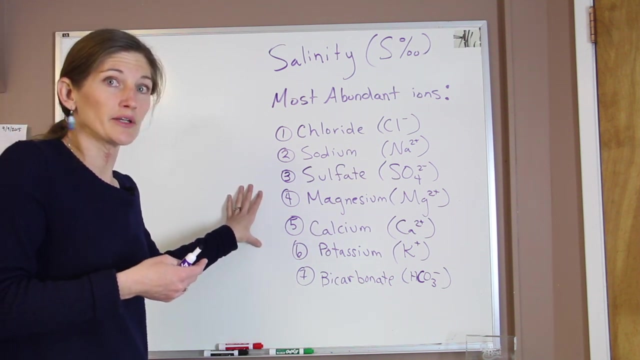 But not all of them are found in our river water. Some of them are active, Some of them are active. Some of them are active. Some of them are actually released through volcanic outgassing, So as the volcano erupts, it's going to be putting out things like magnesium. we'll start to see some sulfate coming out, and that volcanic eruption process is part of where our water came from originally too. 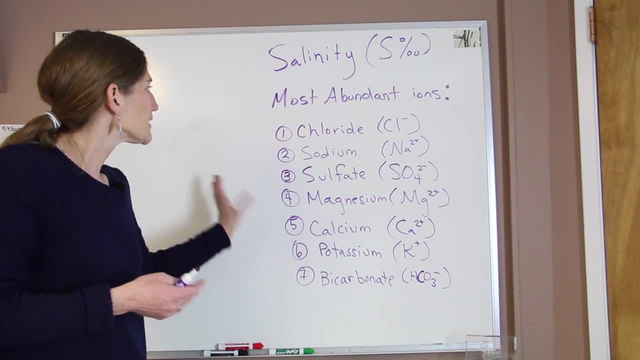 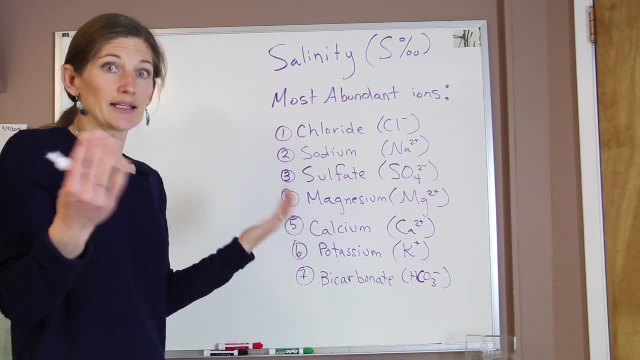 So, with the water vapor and some of these ions, all of that material is getting added into our oceans And you might really easily think that if this is constantly getting added into the oceans, our oceans must be getting saltier over time. But that's not the case. Instead, what we find is that our average salinity over time is constant, So the amounts of salts that we see and the ratio of those different ions in relationship to each other stays constant over time. We have what's called a steady state. We have what's called a steady state, which means that the amount that is added in on average over all of the oceans equals the amount that's removed. So we're left behind with this constant average global salinity of 35 parts per thousand. So the question is: where or how are all of these ions removed? And they're removed by the process of the rock cycle, So we create more sediments. 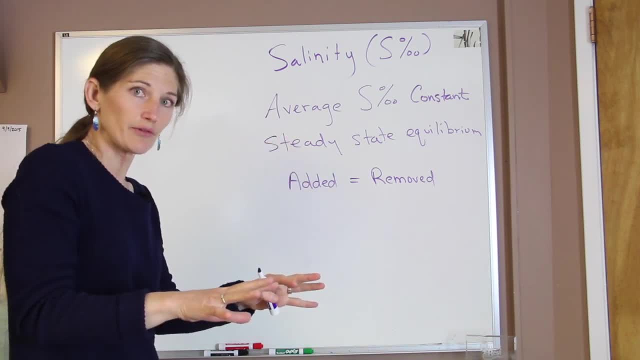 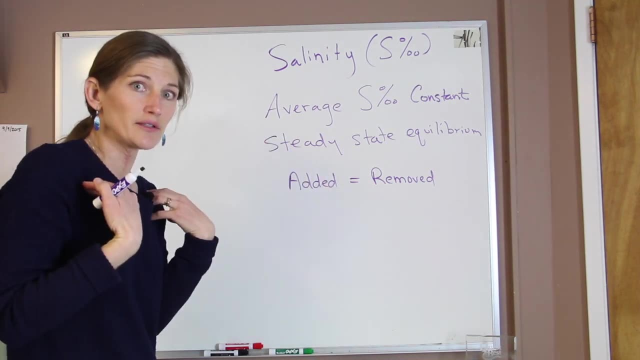 Those ions are going to precipitate out of water onto the bottom of the seafloor. That's one way We do have organisms in the water column that start to pull those ions out of the seawater to make their shells Like our foraminifera. they take calcium and the bicarbonate and they're going to create a calcium carbonate shell. 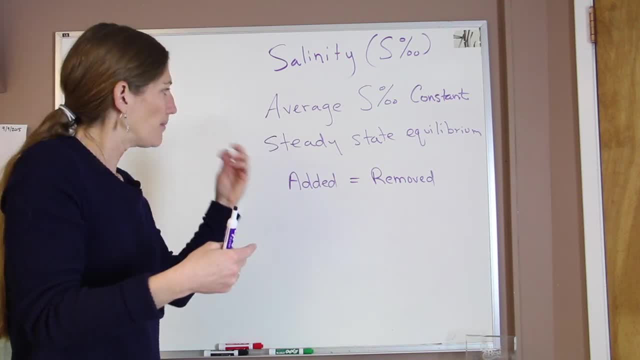 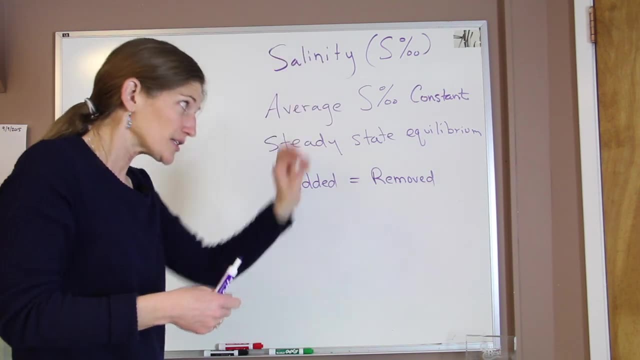 that is in the water column, but it's now no longer part of the dissolved ions. That's another way that we can remove it. Then again, when that organism dies and it starts to sink to the bottom of the seafloor. 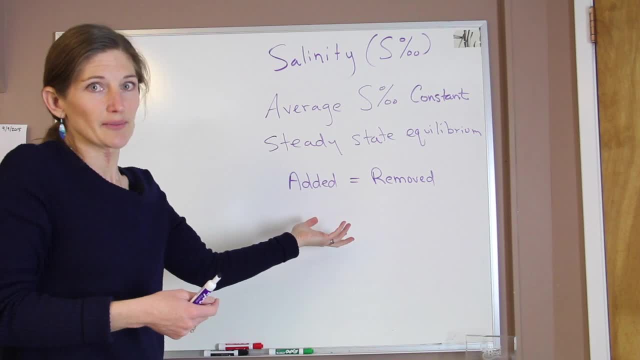 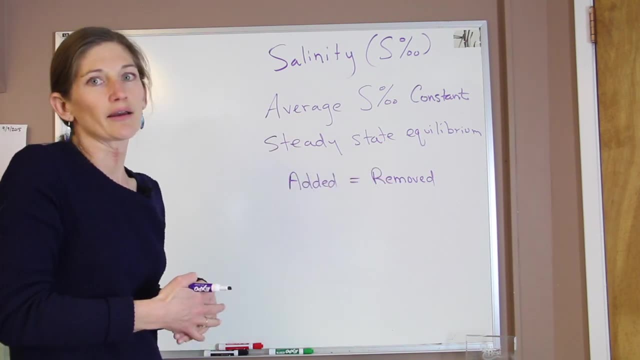 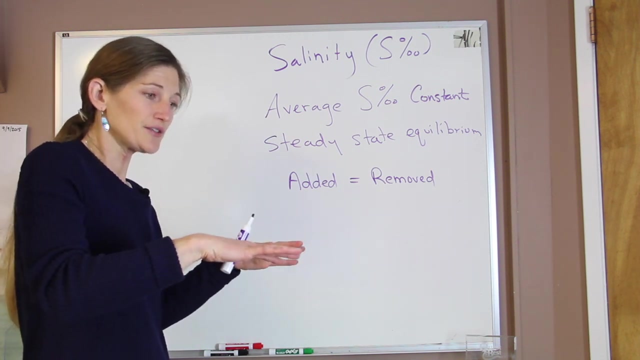 its shell becomes some of those sediments that we talked about. We also have minerals that are precipitating on the bottom of the seafloor, that are removing these ions, And we have plate tectonics. that's happening As the ocean, the oceanic lithosphere, is moving around. it is subducted into our subduction zones. 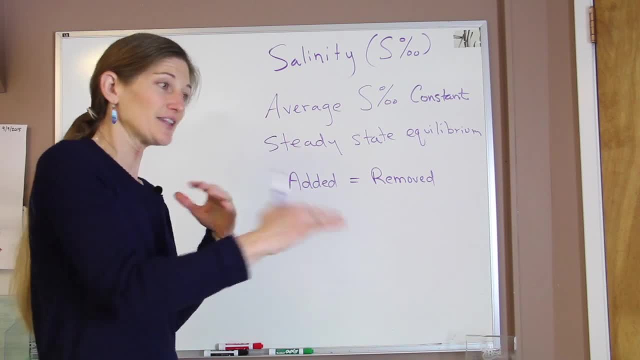 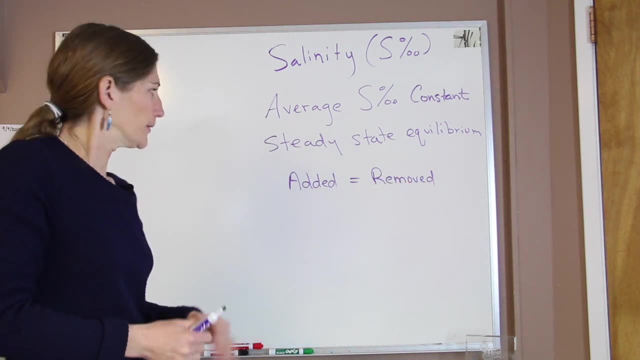 And as it goes down it takes the crust, it takes the lithosphere and all the sediments sitting on top and it starts to wash And then we wedge it down into that subduction zone Again, removing these ions from the seawater. 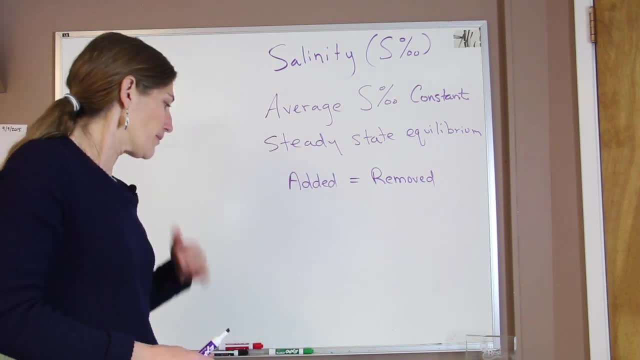 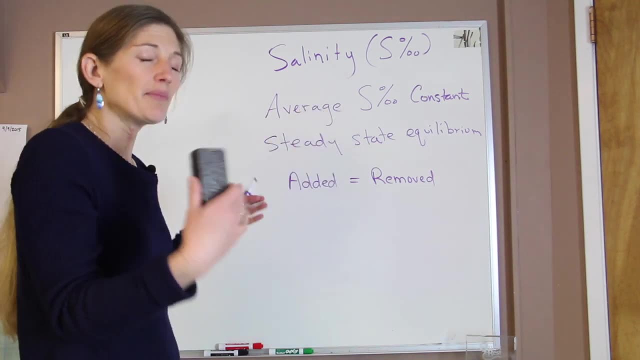 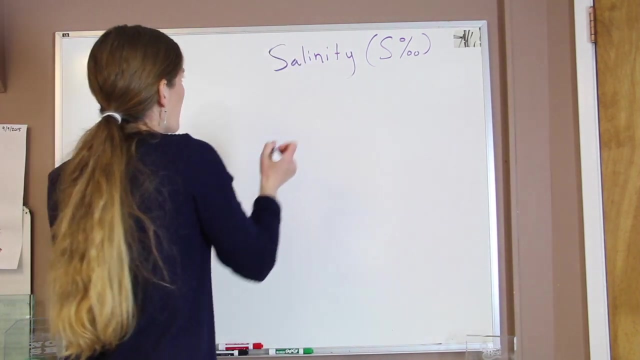 So the amount that is added is equal to the amount that's being removed. We do when we're talking about this. I'm talking about the average ocean salinity, But we do see variations. when we look around our oceans, One thing that we notice is that we have places of lower salinity. 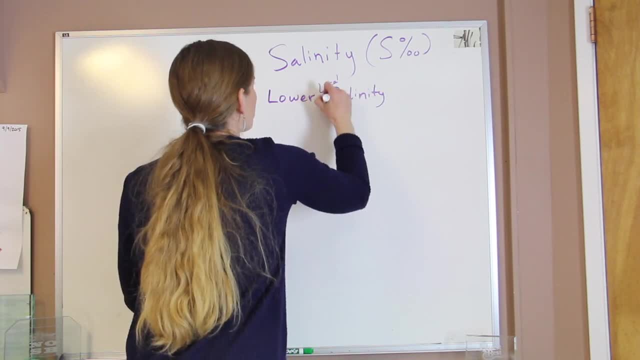 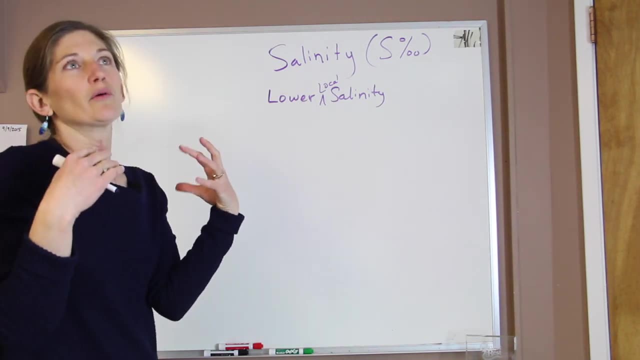 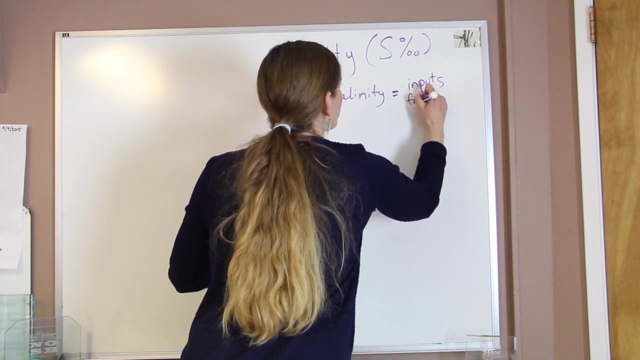 And these are- we'll call it lower lows, And these are local salinity. Okay, Now, when we want to go and understand why we might have lower salinity in a place, we have to think about what makes water salty. This is a place where we have inputs of fresh water. 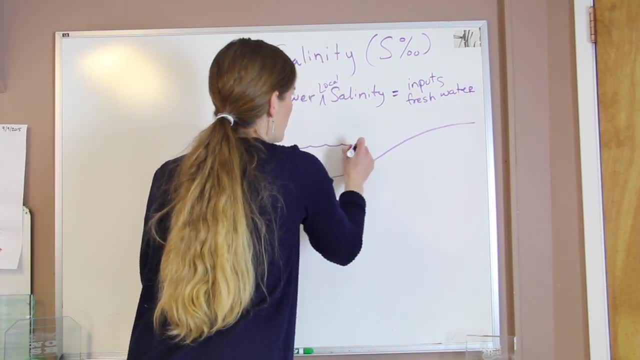 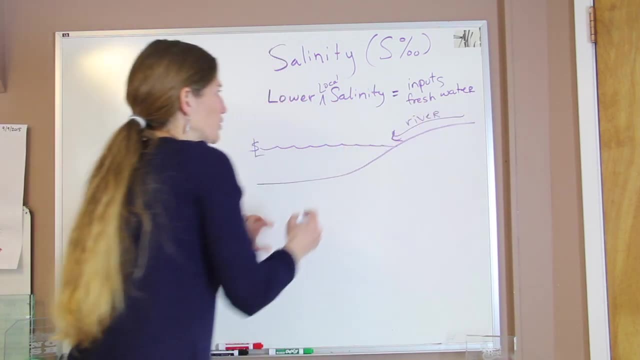 So, if we think about it, the most obvious place that we have inputs this is our sea level, And here we have a nice river moving water into the oceans And as that water comes down, while it might be picking up some ions from weathering, overall, the water is much lower in salinity than the seawater, So our sea salinity at this location goes down Big rivers that have high outputs. lots and lots of water that it's adding into the oceans are associated with these local lowering in salinity. 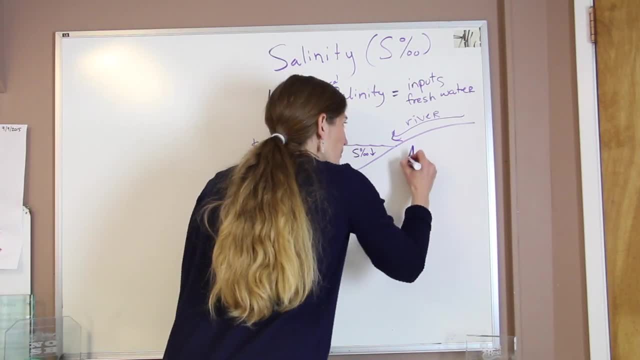 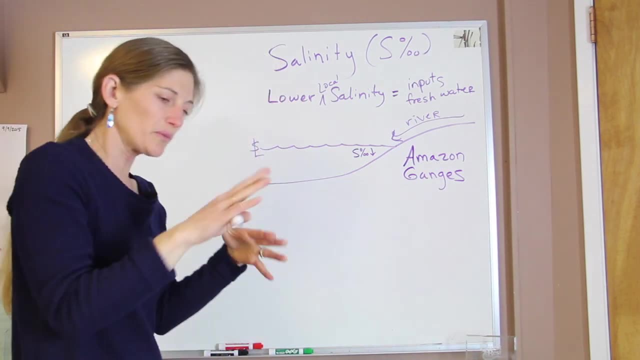 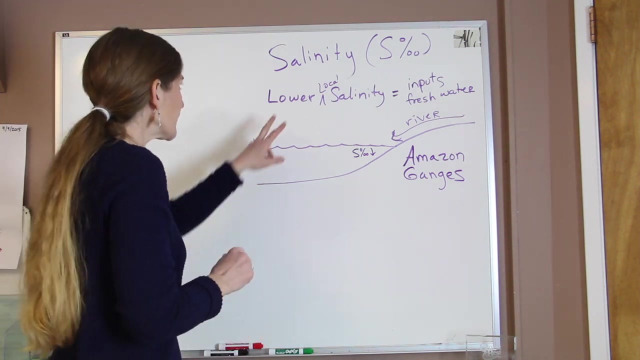 Two big rivers to remember that do this would be the Amazon And the Ganges. Okay, so we do see, when we look at that global salinity map, that right around the mouths of these rivers we see lower salinity In places. another way that we can have an input of fresh water is if we were to 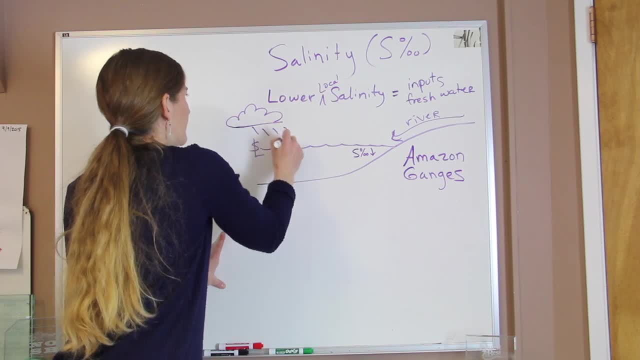 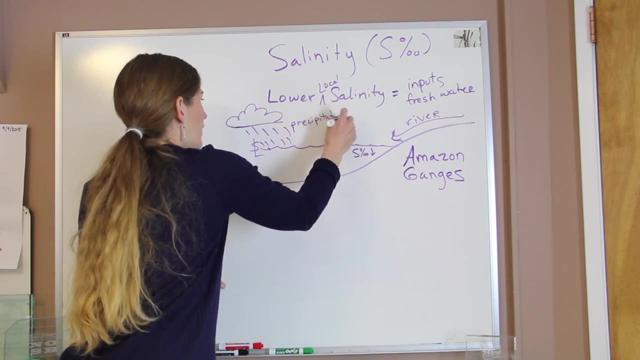 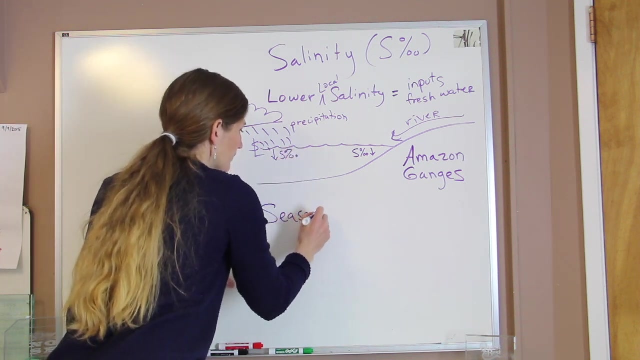 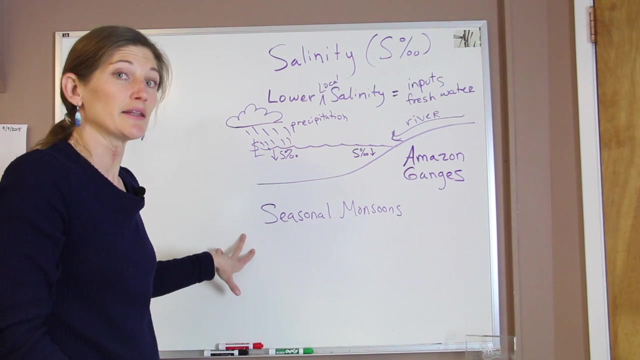 I'll just draw it here: big cloud and we have heavy precipitation. That's also going to lower the salinity in that area. Our seasonal monsoons lead to a lowering of the salinity in the places that they occur. One place that's really apparent is in the Bay of Bengal. 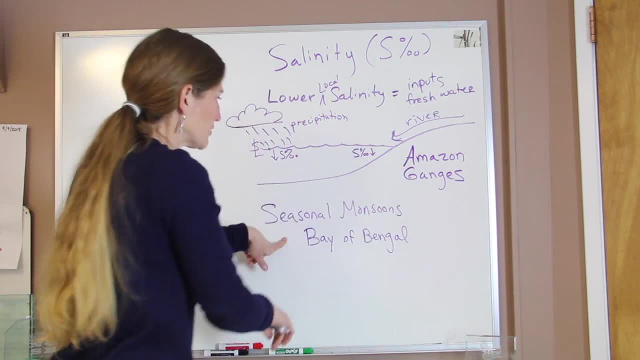 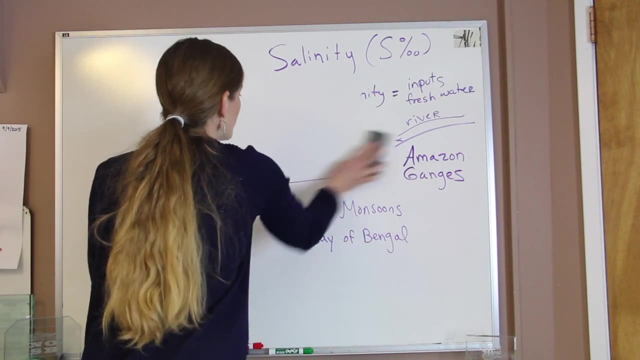 So we have addition of seawater and also these monsoon rains, so we see definitely a lot lower salinity, Yeah, in this area. Now the next thing we would want to understand is: well, where is the high salinity? Where is that going to be? 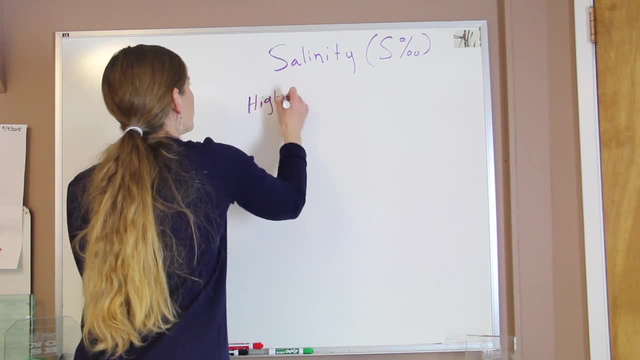 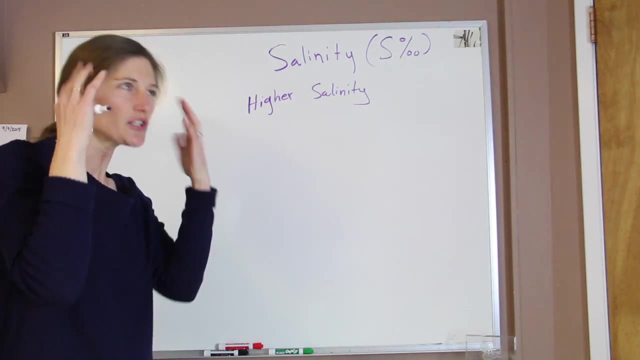 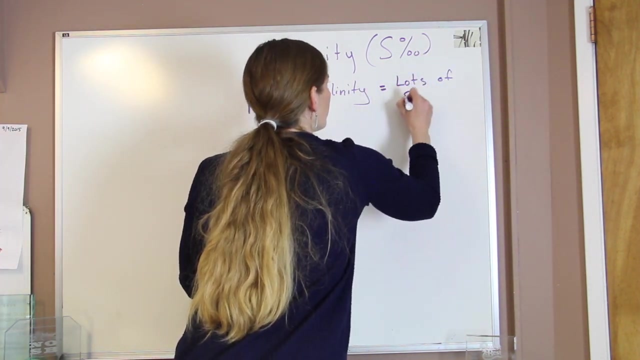 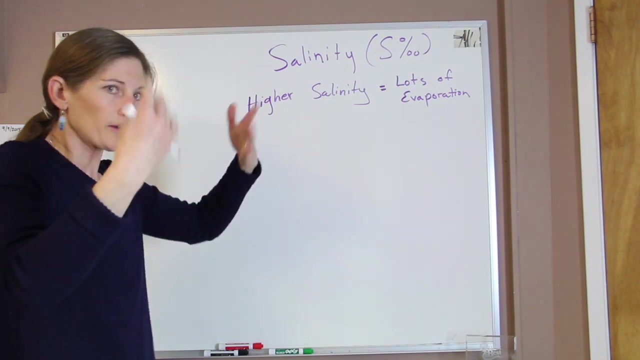 Because we do certainly find higher salinity areas, And in order to understand why we would have higher salinity, we need to just think about the process in reverse. These are places where we see lots of evaporation, So as we start to evaporate water out, all the salts get left behind. 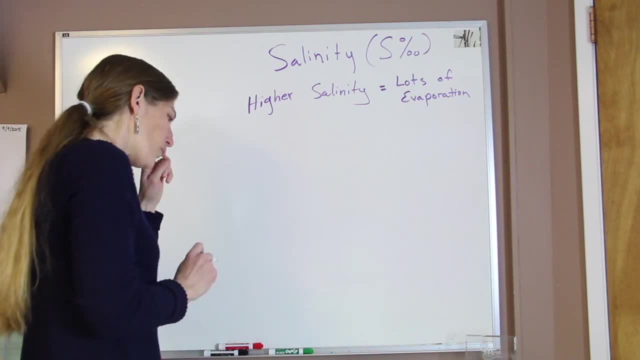 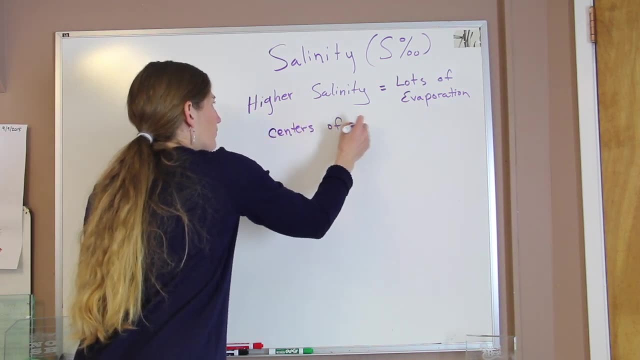 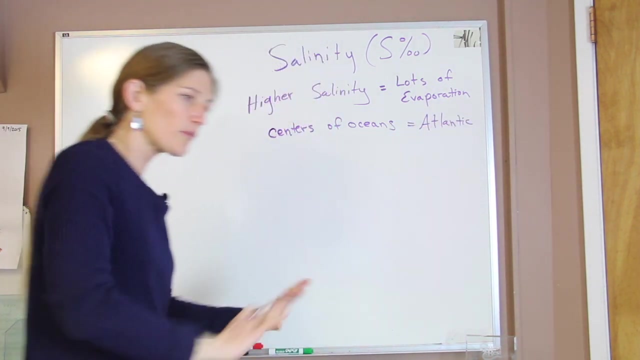 so our salinity in that area is going to be higher. One place that we see this happening is in the centers of our oceans. They are, in general, higher than others, especially in our Atlantic Ocean. So the waterway out there it's isolated, doesn't have lots of precipitation. 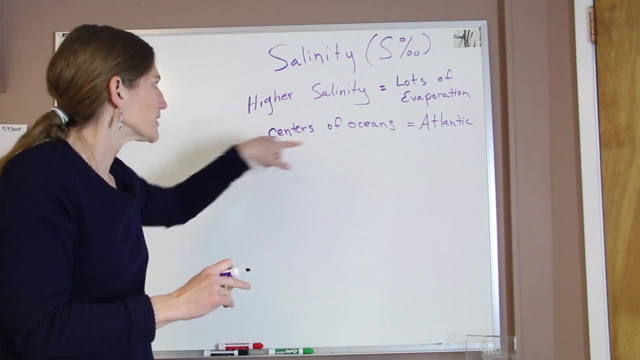 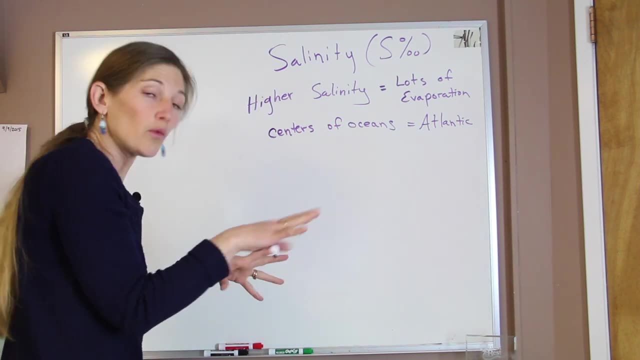 and we're going to start to see more evaporation leading to more salinity, Kind of in the middle of our ocean basins, Another place that we see it are in kind of these more isolated water bodies. So if you were to think about- let's see- Gibraltar. 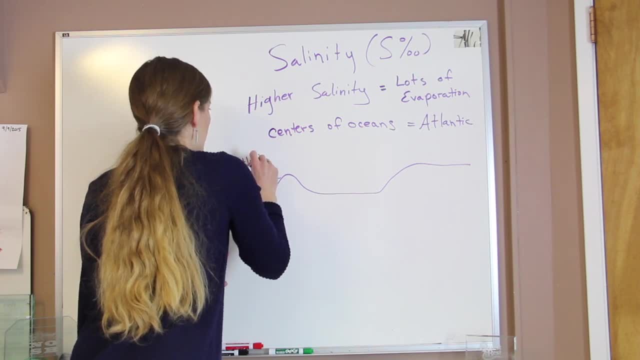 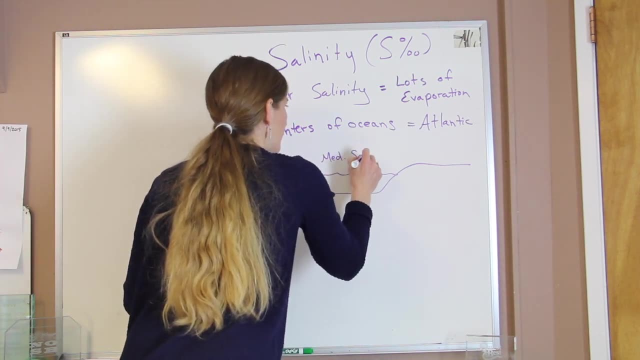 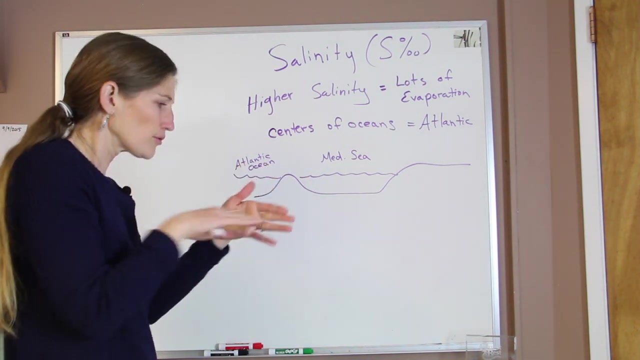 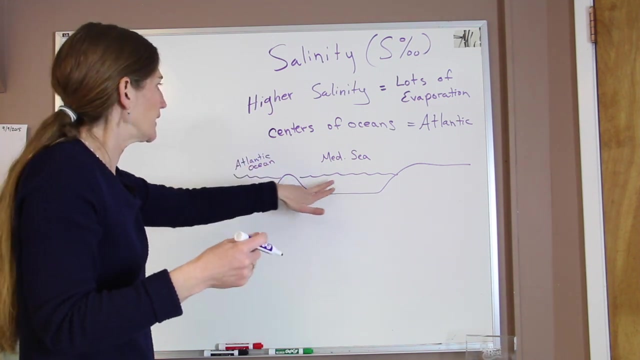 Here we have. this is our Atlantic Ocean And this can be our Mediterranean Sea. In this area the Mediterranean Sea is pretty isolated. Water does flow in and out through Gibraltar into there, but it's actually not a lot. So the Mediterranean Sea becomes more isolated. 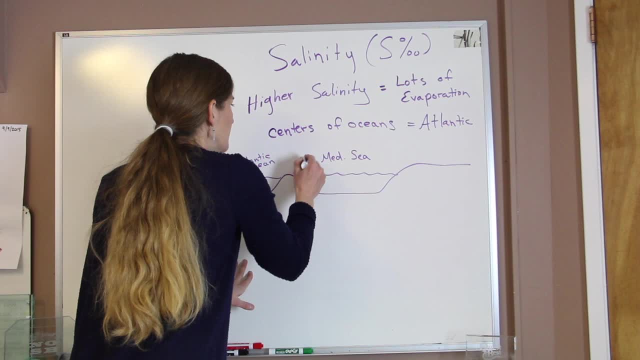 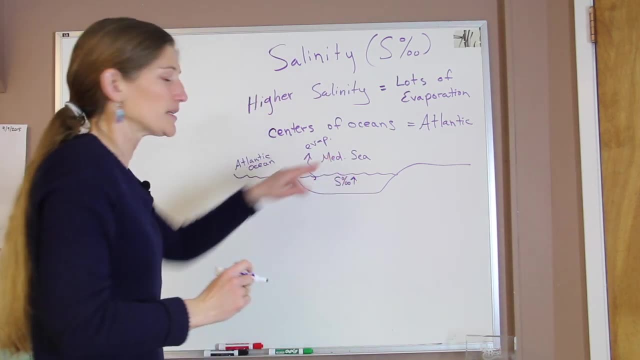 As it's isolated. warm temperatures, we're going to start to see evaporation And that's going to lead to an increase in the local salinity. So the Mediterranean Sea is much higher. Another place that we see this same process happening would be in the Arabian Sea. 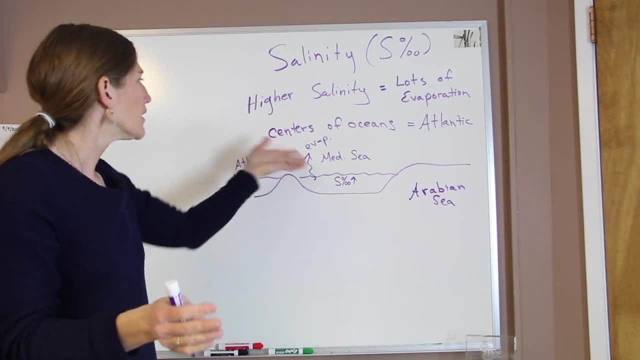 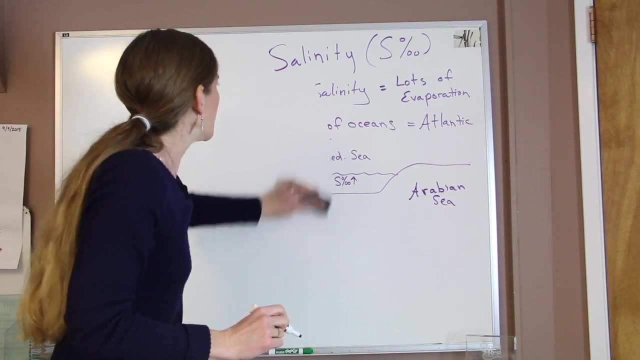 Again, places where we don't have as much input of fresh water, we have lots of evaporation, So we see higher salinity getting left behind All right. Now the one that I wanted to talk about in discussing local changes in salinity. 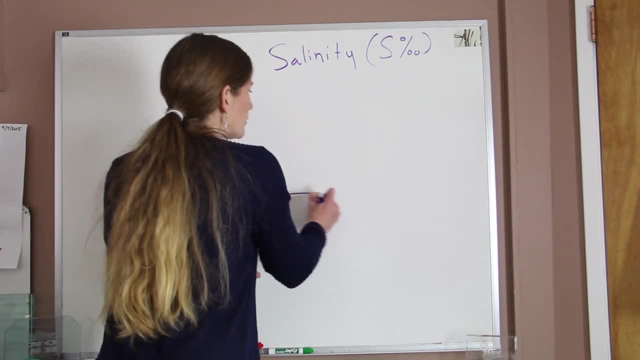 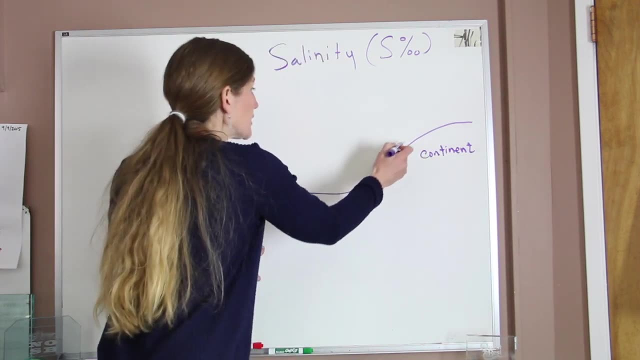 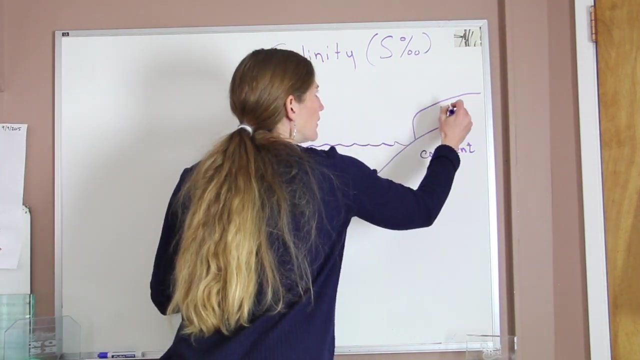 is the role of sea ice. So if we would just go and we draw in our continent And we can say that this is Antarctica, We have our sea level, And then we'll just imagine that we have a big block of ice, Our glacier is sitting there.